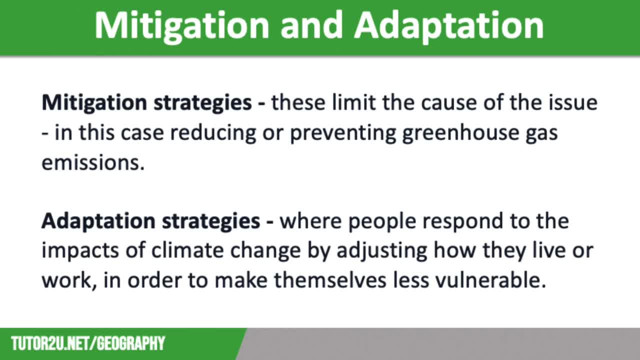 in order to make themselves less vulnerable. These strategies are local, as they respond to localised impacts: for example, building homes on stilts in areas where there's no climate change- This can be an increase in flood risk- or planting drought-resistant seeds in areas of low rainfall. 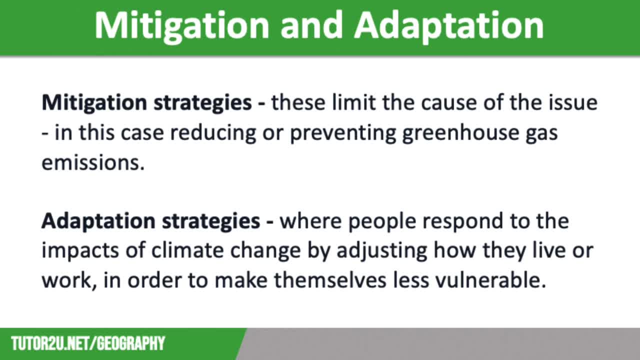 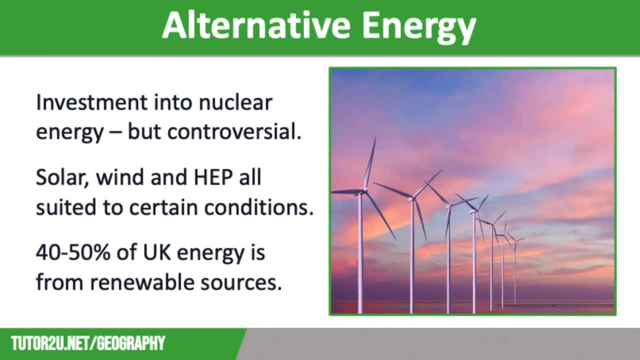 This video focuses on climate change mitigation. We will have a separate video for adaptation. Our first mitigation strategy is alternative energy. As the populations grow and economies develop, there is an increased demand for energy to fuel domestic appliances, transportation, food production and industrial output. 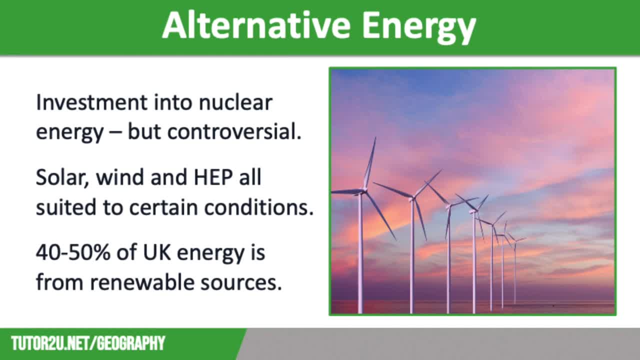 Much of this energy is created by burning fossil fuels, which release CO2 into the atmosphere. As countries sign up to climate agreements, they are using alternative sources of energy. Many countries have invested heavily in nuclear energy. This uses uranium to generate electricity through the process of nuclear fission. 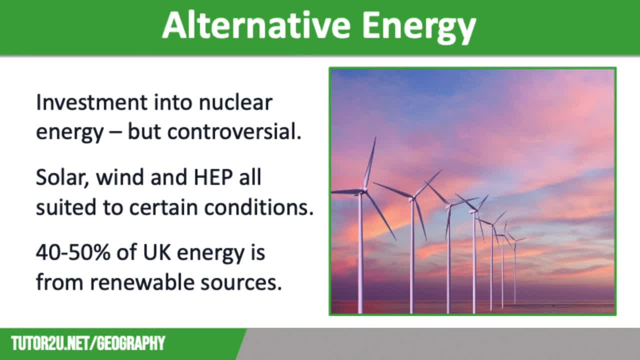 It doesn't emit CO2 during energy production, so it is considered much better for the environment. However, it is extremely expensive and many argue that the risk of radiation leaks or nuclear meltdowns make it unsafe. There has also been an increased investment into renewable energy sources. 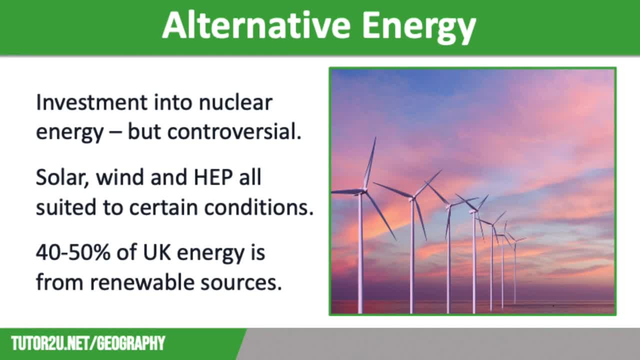 These will not run out and they do not emit CO2 during power generation due to solar, wind, hydroelectric power and geothermal. Currently, renewable energy sources are more expensive than fossil fuels and they can be unreliable. For example, solar and wind power are dependent on the weather conditions. 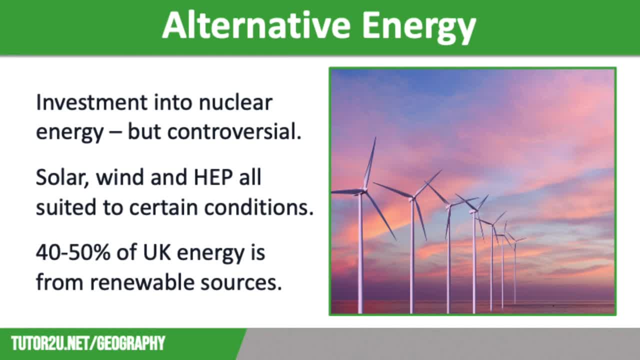 However, there are certain locations ideally suited. Solar panels are great for low-income countries that experience long hours of sunshine, particularly in desert regions. Wind farms are suited to countries with long stretches of coastline, so they can be placed offshore, where the wind speeds are higher and fewer people will oppose. 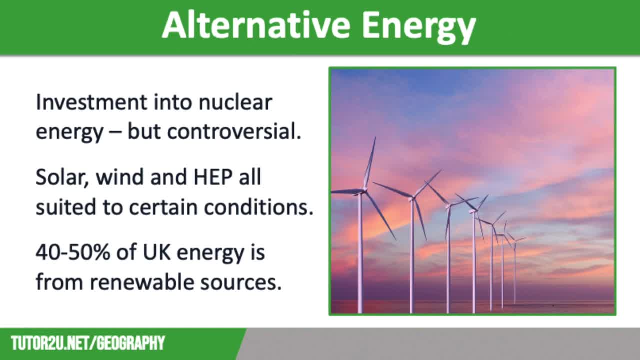 Hydroelectric plants are suited to highland areas with deep valleys and high rainfall totals, giving ideal conditions to build dams and reservoirs. The UK government set a target of 15% of its energy to come from renewable power by 2020.. This has been regularly exceeded for several years. 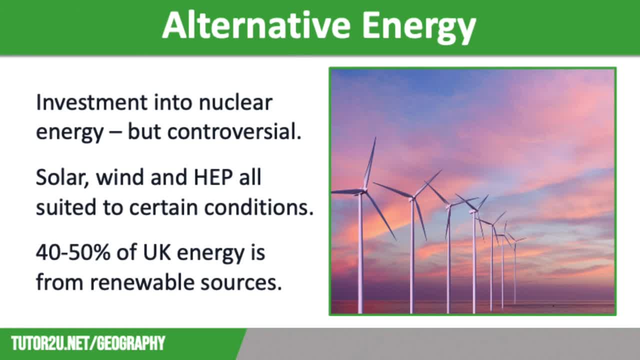 It is actually usually between 40% and 50%, although this does vary on a daily basis depending on weather conditions. The biggest share of this is wind power, which accounts for around 40% of UK energy. This is down to the huge investment into offshore wind farms around the UK. 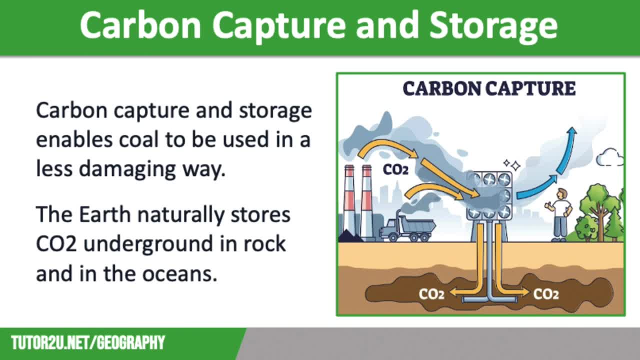 Our second mitigation strategy is carbon capture and storage. Coal is the most environmentally damaging fossil fuel. Unfortunately, it is still widely used in electricity generation across the globe, particularly in newly emerging economies. China gets 69% of its energy from coal and India gets 79%. 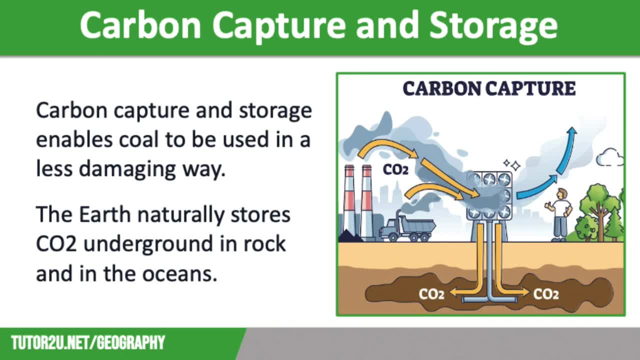 However, in the last decade, the US's share of energy from coal has gone down from 50% to 20%. Carbon capture and storage enables coal to be used in a less damaging way. The Earth naturally stores CO2 underground in rocks and in the oceans. 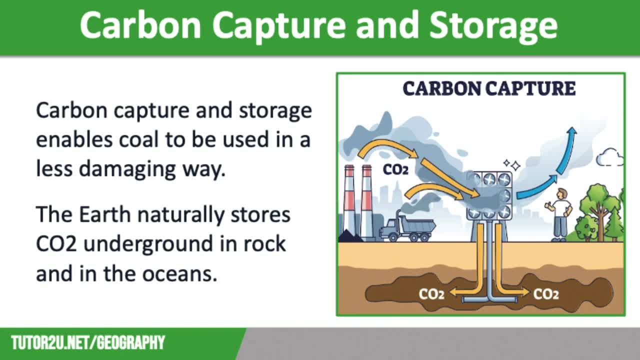 By using technology, it is possible to capture our energy. This means that it can store up to 90% of CO2 emissions from generating electricity and industry. This gas is then compressed and transported by a pipe into an injection well and injected into the ground where it can be stored, as you can see on the screen. 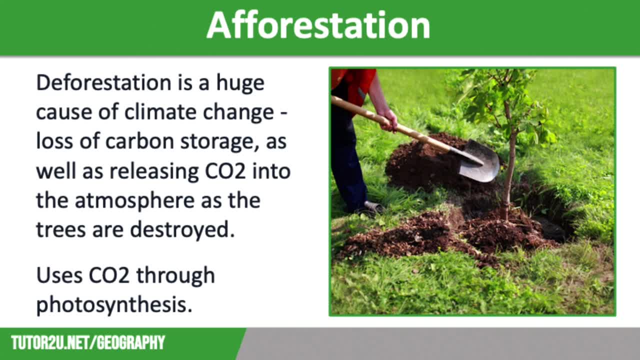 Our third mitigation strategy is afforestation. Deforestation is a huge cause of climate change, Loss of carbon storage, as well as releasing CO2 into the atmosphere as trees are destroyed. Planting trees reduces the amount of CO2 in the atmosphere through the process of photosynthesis, converting it into oxygen. 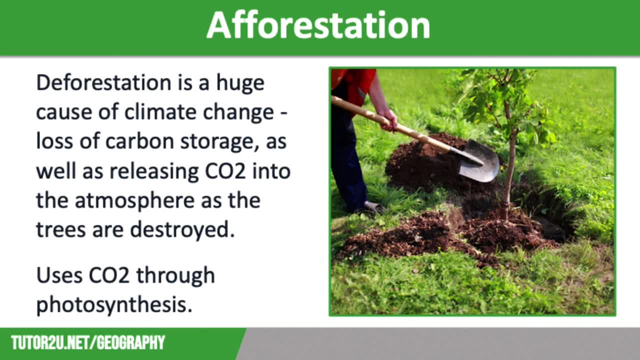 Trees also release moisture into the air through transpiration. This cools and condenses to produce clouds, which reduce solar radiation. There are also other benefits of afforestation projects, such as increasing biodiversity and reducing the risk of desertification, For example, through the Great Green Wall that has been planted. 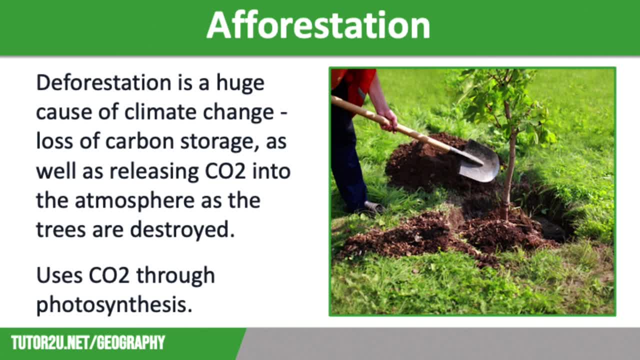 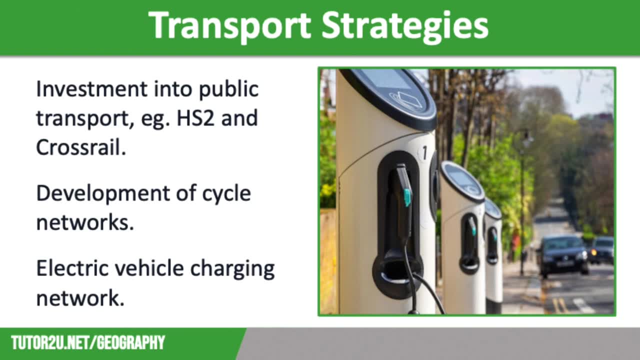 right across the Sahel region in Northern Africa. Our fourth mitigation strategy is lowering emissions from transport. Countries like the UK are investing heavily into public transport to reduce the number of cars on the road, which would reduce the amount of CO2 emissions from transport. 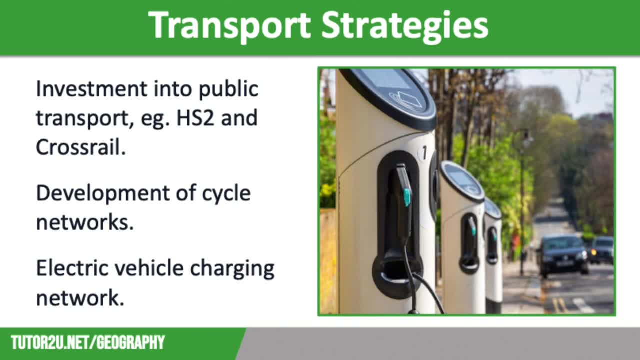 Huge infrastructure projects include the High Speed 2 rail link linking London to the north and Crossrail, which has improved rail links across London. These projects will also benefit the UK economy. London also has the congestion charge and the low emissions zone to reduce car usage across the city.